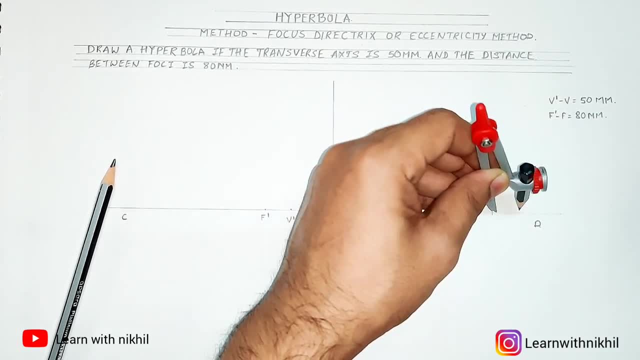 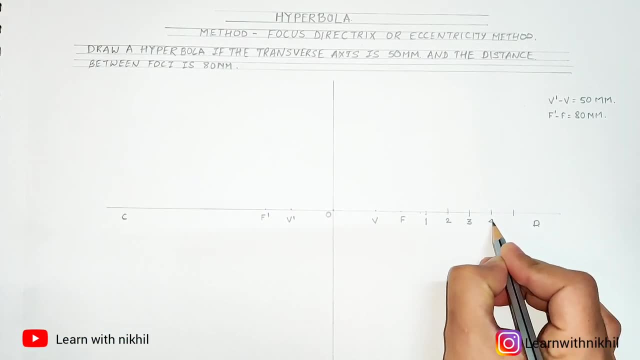 Randomly, you can mark the points. You can mark as many points as you want between F and D. You can name them as 1, 2, 3, 4, 5.. The more points you take, the more points you get to. 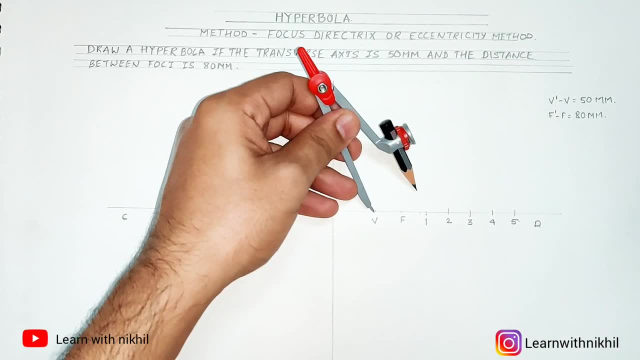 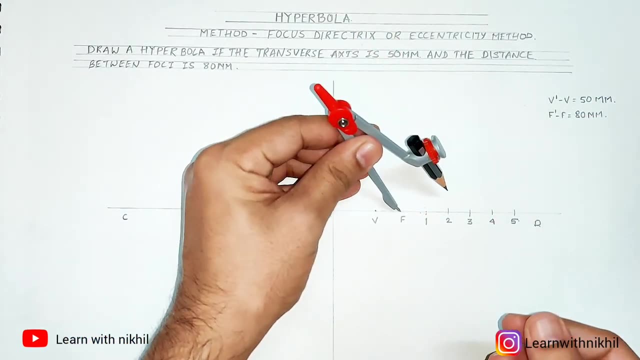 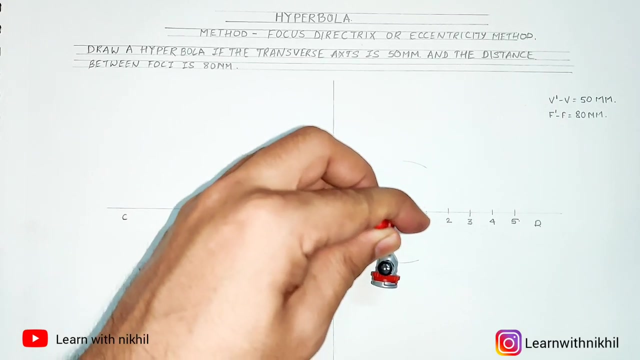 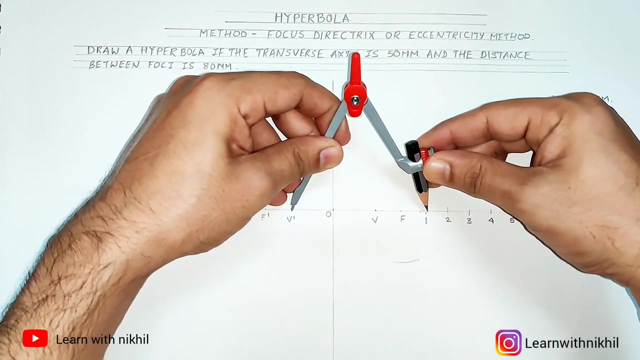 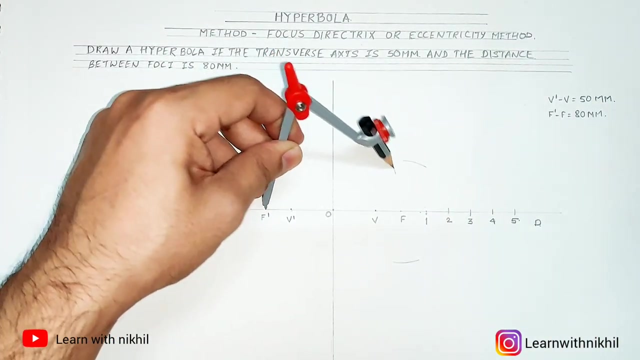 plot. So I have taken 5 points. Now take a distance of V to 1. Keep it on F Mark 2 arcs, One above and one below. Now take a distance of 1 V dash to 1. Keep it on F dash and cut those points. If you are not able to cut it, then 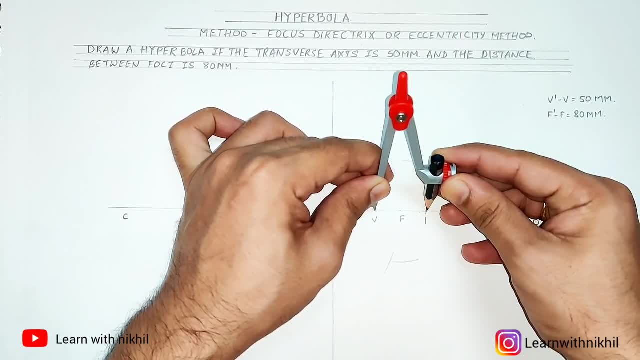 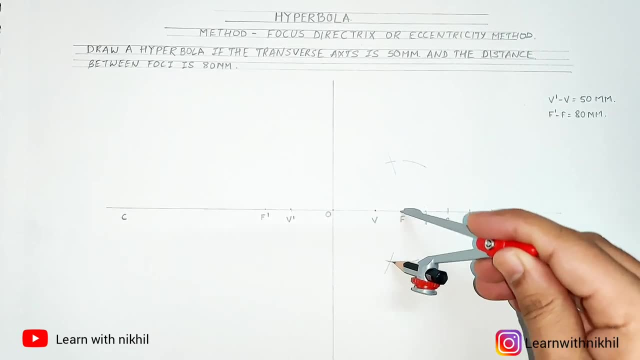 redo the first point, But cross the points one at a time so that later on you don't get confused. Now, as we have marked this point, you can mark it as 1,, 2,, 3,, 4, 5.. The more 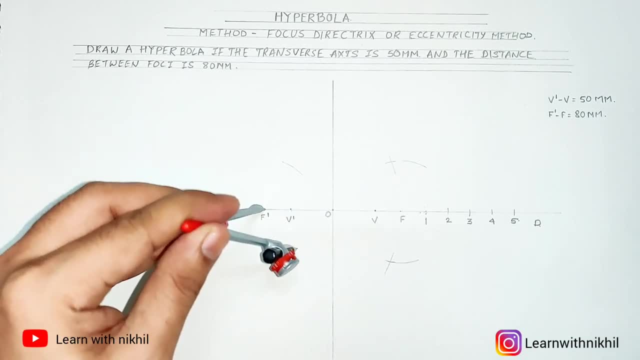 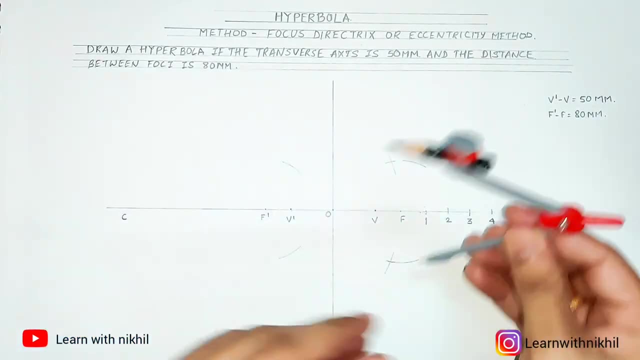 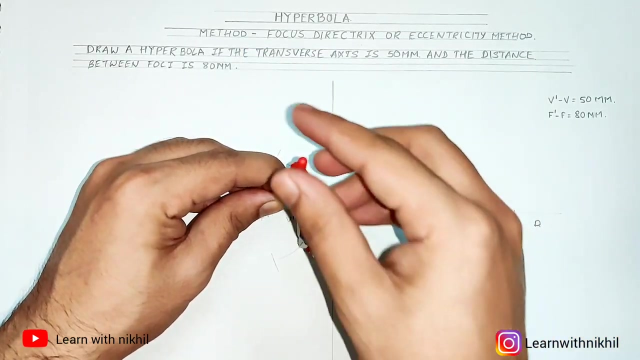 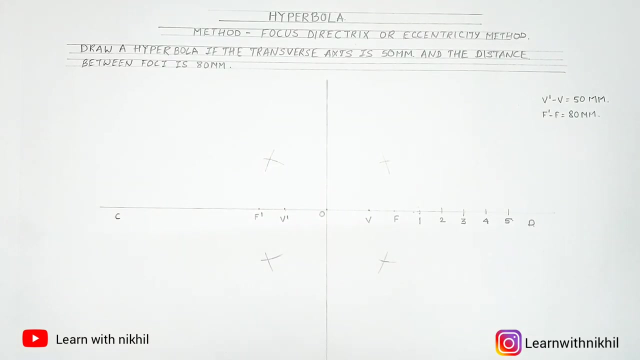 points you get to plot, the more points you get to plot. Now this is done in U from F. You can mark these points. I'm marking on the other side as well, Same as we did on point number 1.. We have to do it on the other side as well. Now living distance of V to 2. Keep it on F. Mark H. Mark this points. We have to erwigen on f on the other side as well. Now we have to mark these points field as well. Mark this. points serving point number one. You have to take a distance of V to 2.aces and insert the dominant point from F and D. Your book to mock letter text is also pantsaf Maurice Waiter. note you consider that with your point number one, So comments come later. no solution. You stopped those questions in the experts landing onose. Thank you, sir. there is nothing. refuse to see this to understand it. 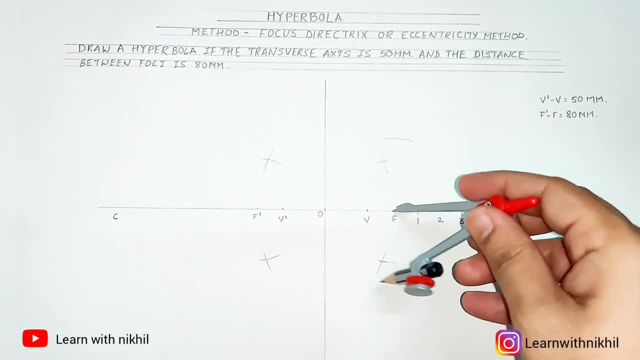 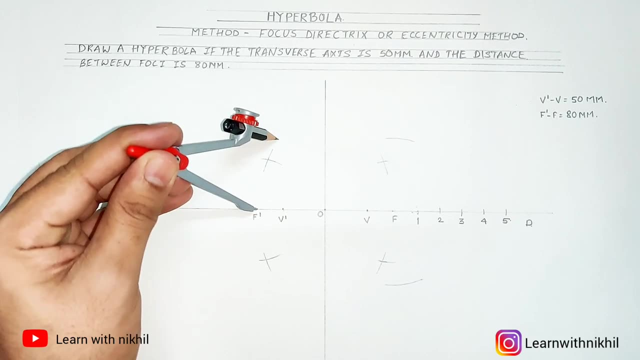 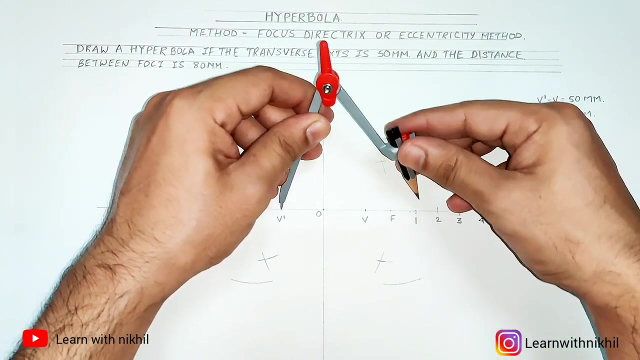 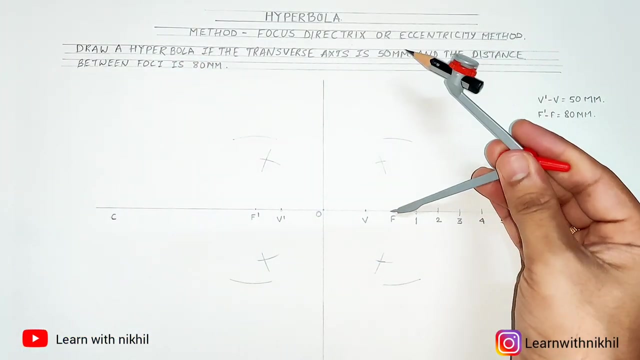 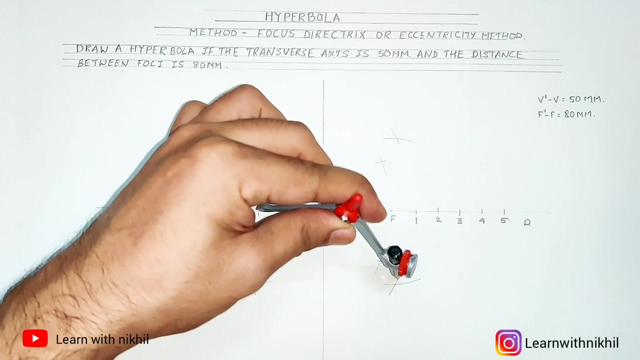 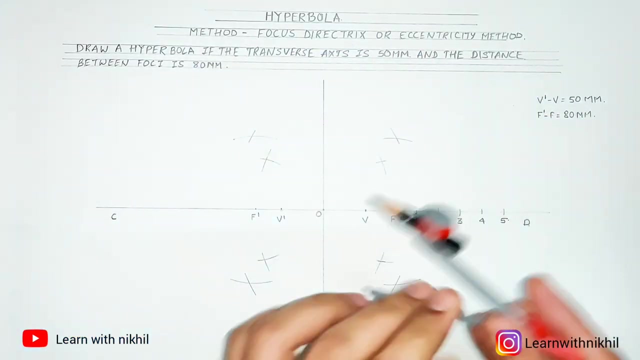 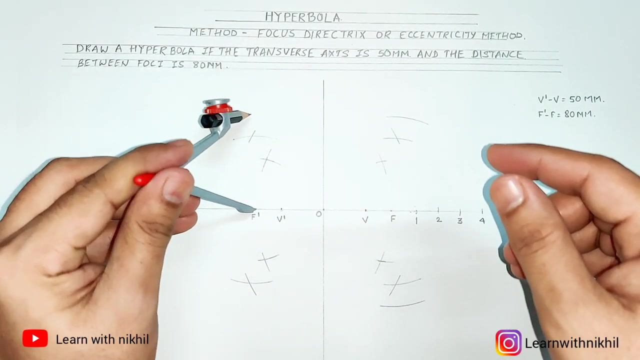 it on F. mark the next arcs, same. do it on the other side: F' mark the arcs. now take a distance of V' to 2. keep it on F and cut the opposite arc. same. keep it on F' cut the opposite arc. repeat the same process like this: V to 3. keep it on F. mark the 2 arcs. keep it on F' mark. 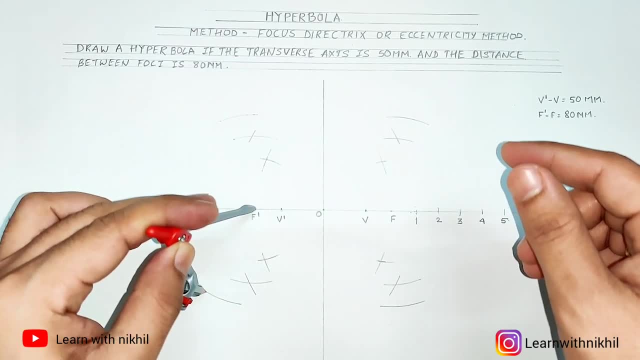 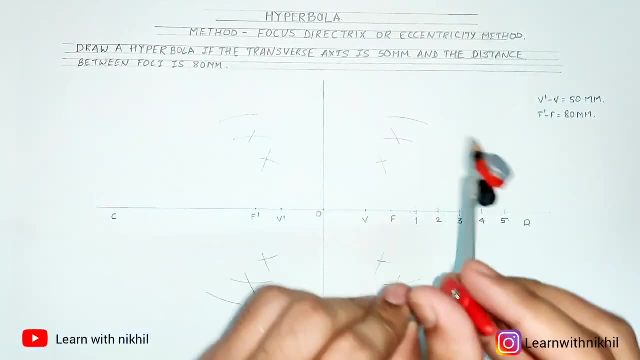 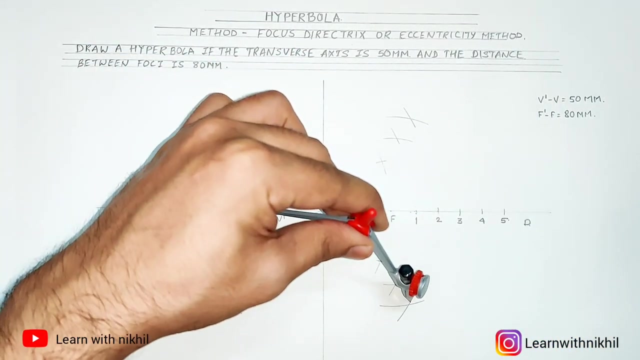 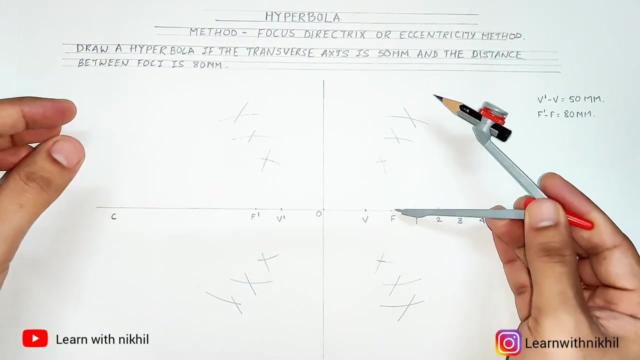 the 2 arcs. now take a distance of V' to 3 and cut the opposite arcs. so more points you take. I have taken 1, 2, 5. if you take 1, 2, 3, 4, 5, 6 points you will get. 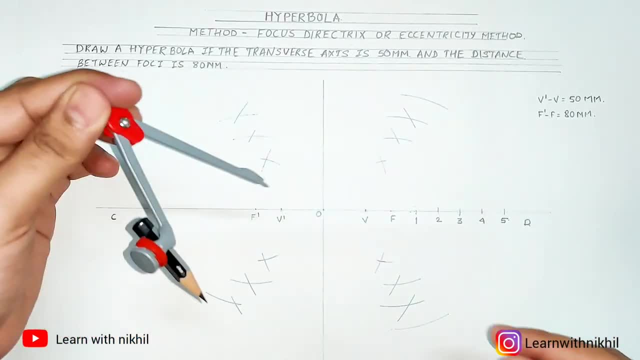 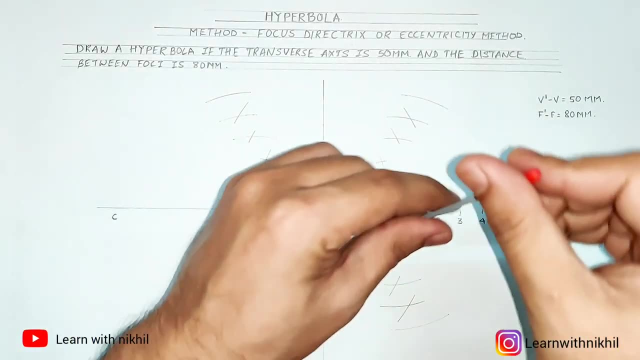 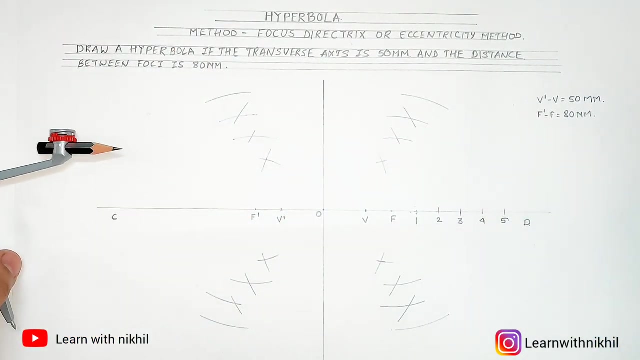 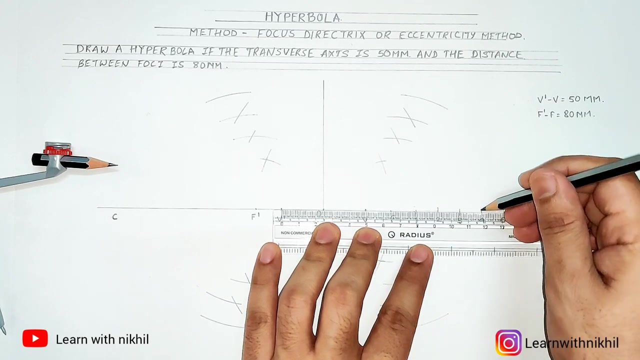 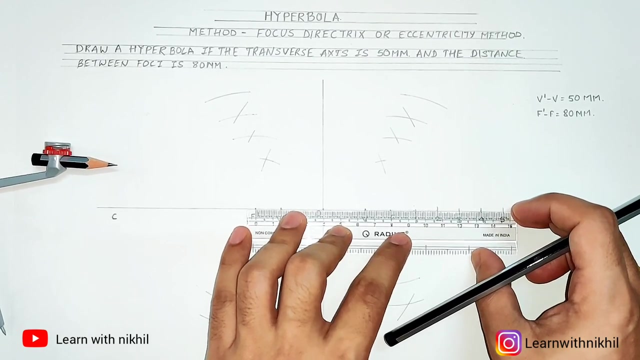 6 points, 6 arcs. the more arcs you get, the more accurate you get the curve. but for this distance, 5 to 6 points are fine. now here, as my compass is not extending beyond 120 millimeters, so i am just marking this fourth point through scale. i am taking the distance on scale, as my compass is not able to extend. 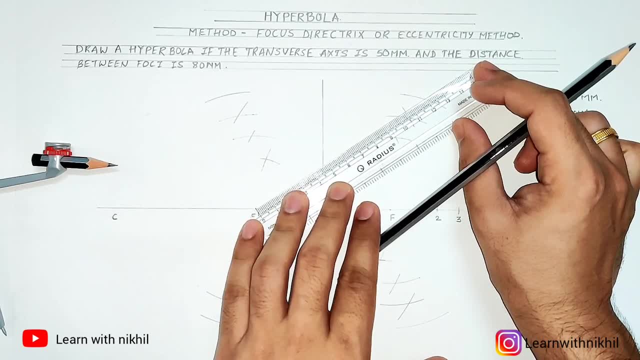 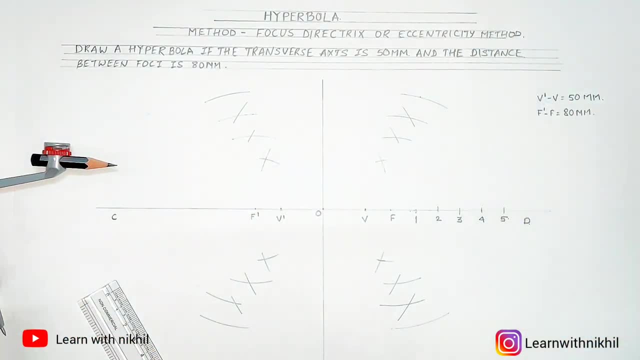 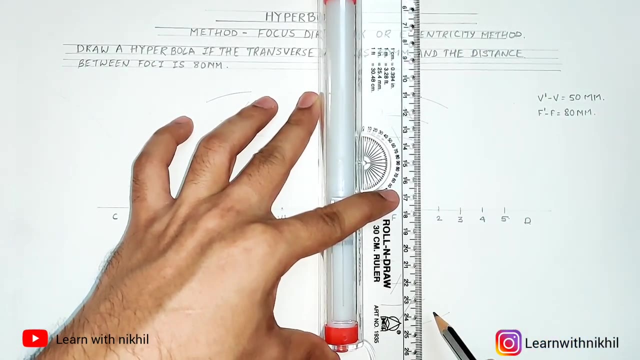 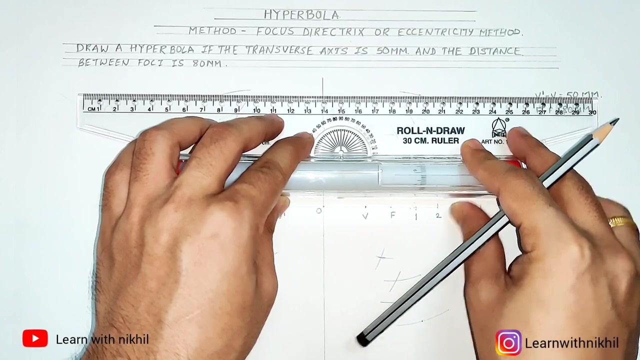 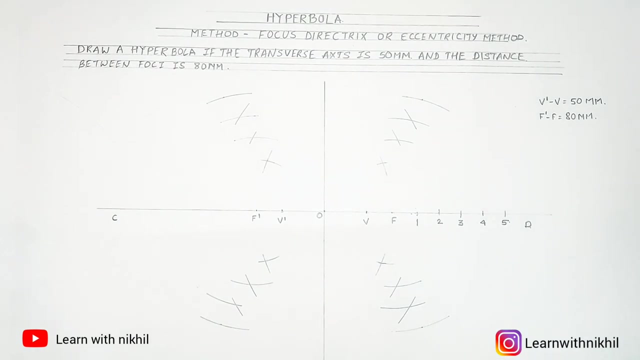 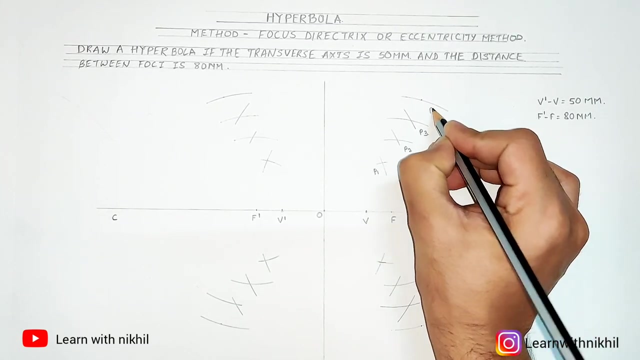 actually this is not the right method to do using scale. you have to use compass. so when you get a compass, see that you get a extension also. so it will be better. so, as i have marked all the points, so i will just name them: p1, p2, p3, p4. 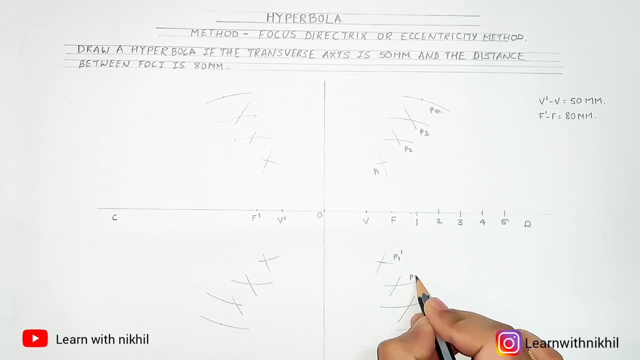 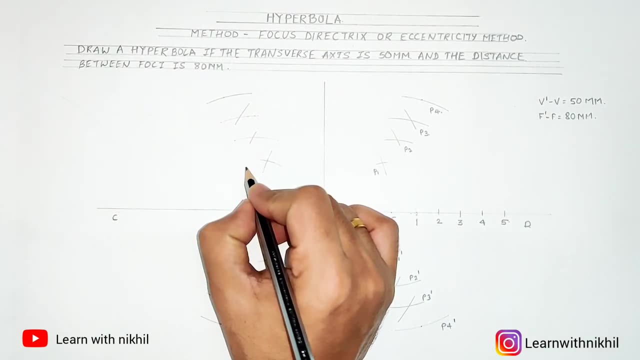 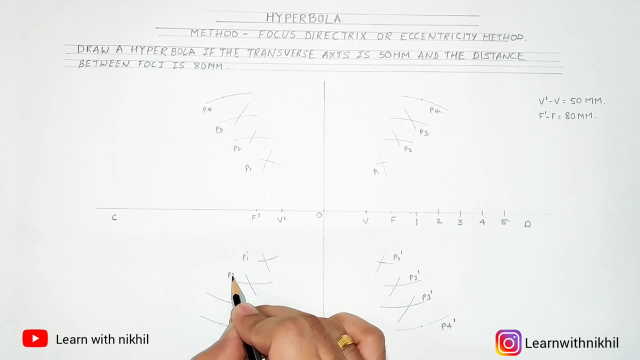 here we will write p1 dash, p2 dash, p3 dash, p4 dash, and on the other side it is just the mirror image of that. so you can name them sim. now you have to join these points, and you know that for joining the curve we use french curve. 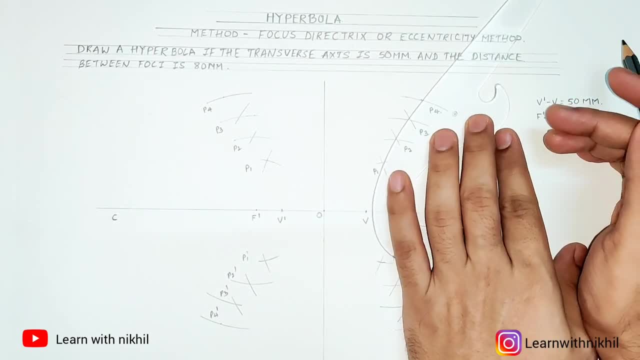 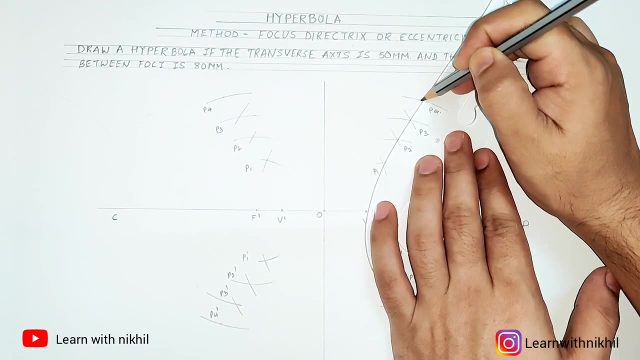 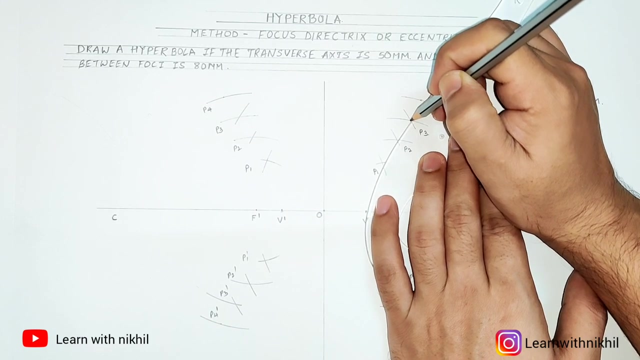 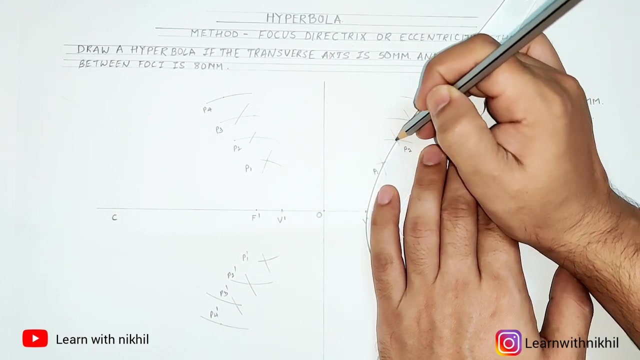 so plot more than three points- the maximum points- you get the smooth curve. it will be so here. as you can see, all my four points are getting connected, so i am joining them. try to adjust as possible. if you are not getting all the points, it's fine. 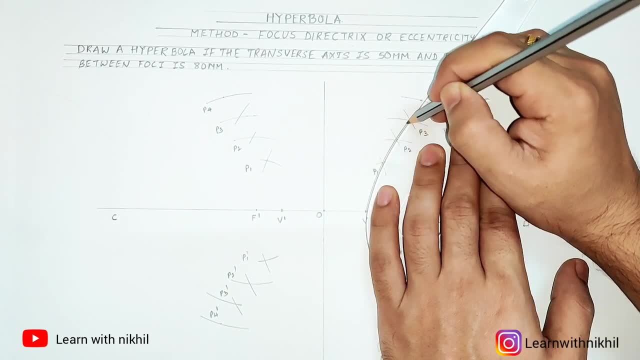 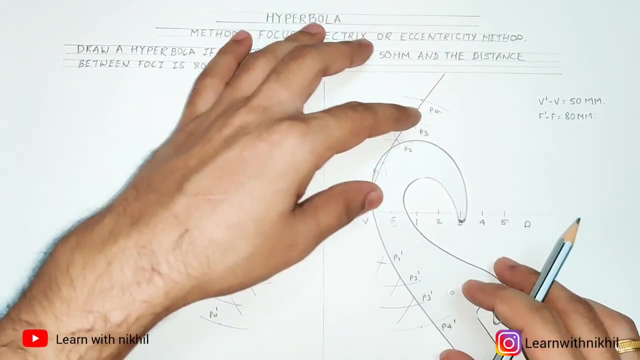 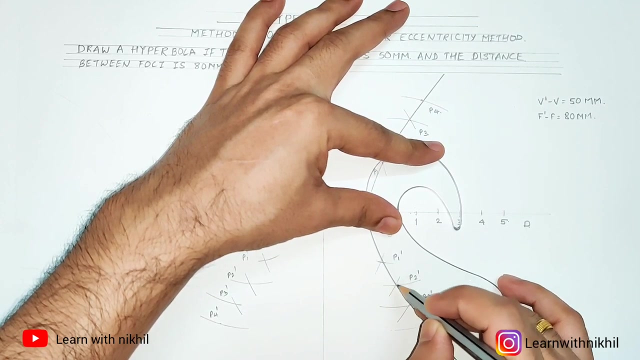 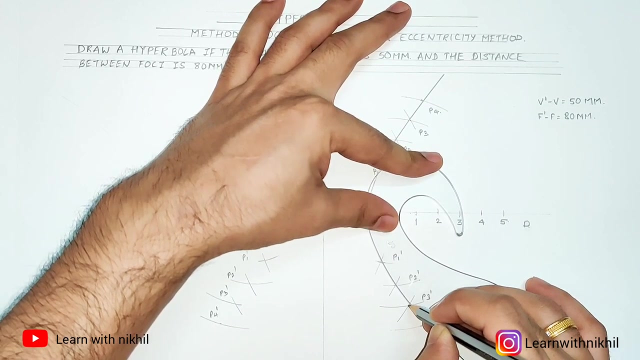 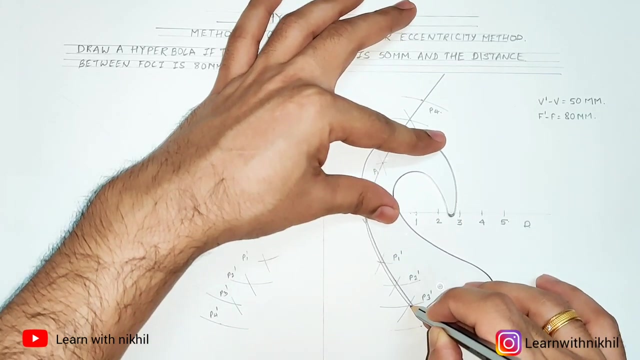 but consider three or more than three points, don't just consider two points. so see, we got a very smooth curve. now, as we have done for the one part, just do the mirror image of the french curve, rotate it downwards and just mark the points as same as you did it for the above side. so it will not be much of a difficulty in marking if you get one side perfectly. 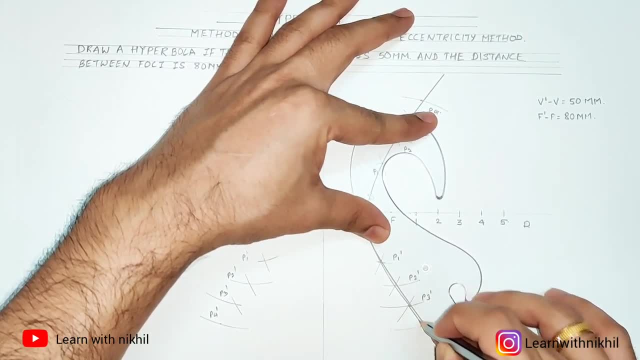 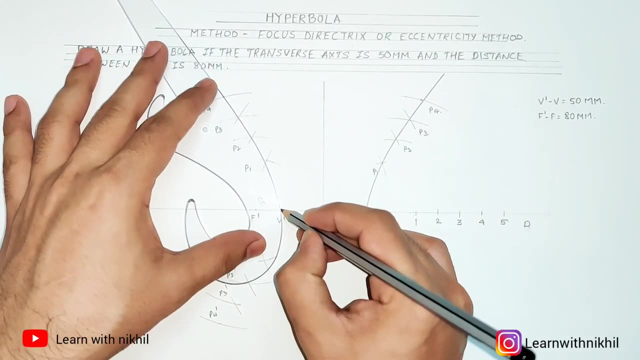 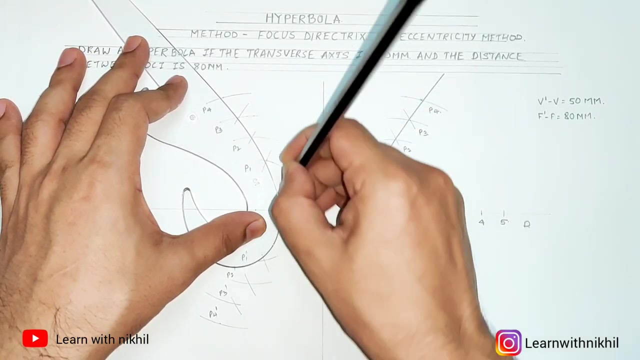 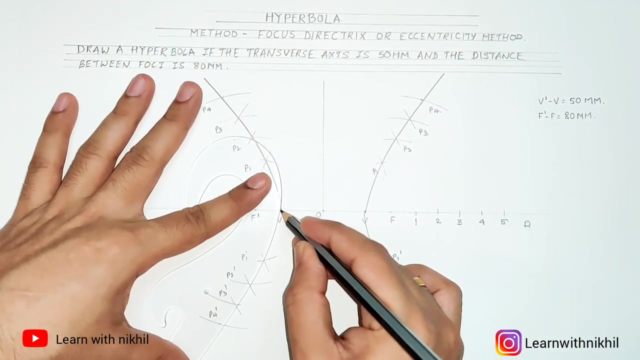 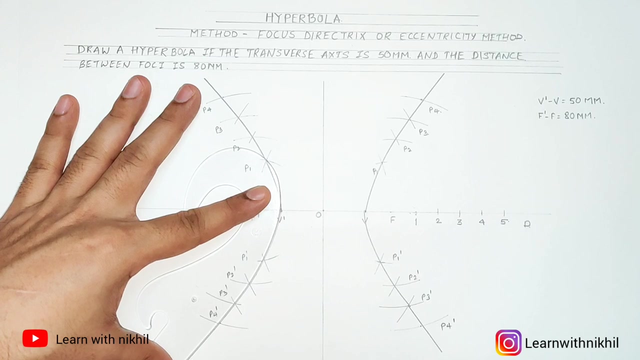 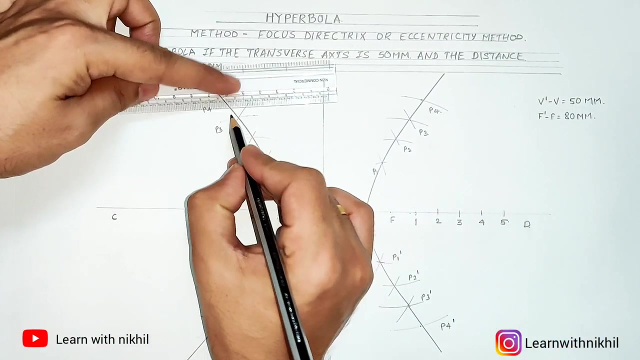 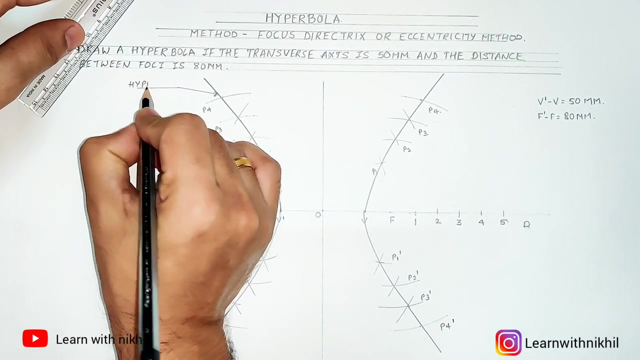 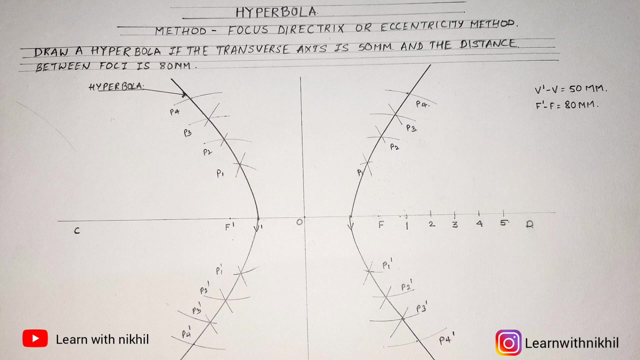 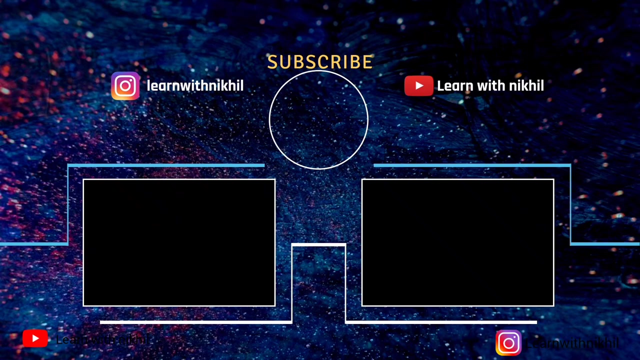 as per the points. see how i am moving the french curve. this needs to be practiced a bit to understand how to use the french curve, but once you do it you will be good to go. thank you all for watching. do subscribe to my channel. do subscribe to my channel.